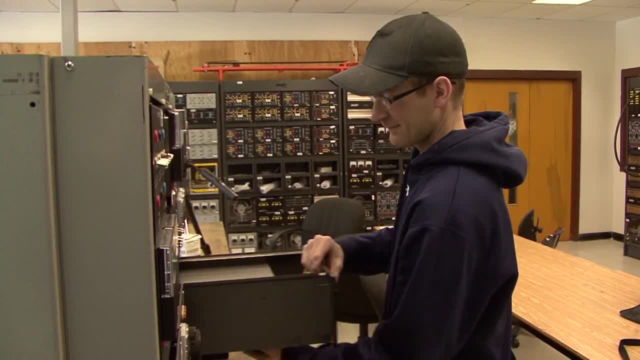 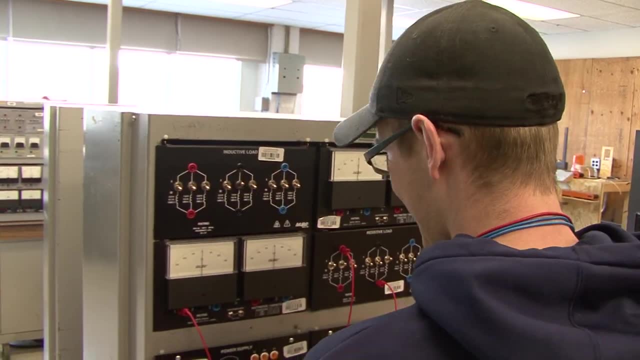 going to happen and get a job in the power and controls field. Like I said earlier, electricity is everywhere. I mean the job possibilities are endless. I guess you would say This is a co-op program. There's two work terms. Right now I have a work term coming up in June with 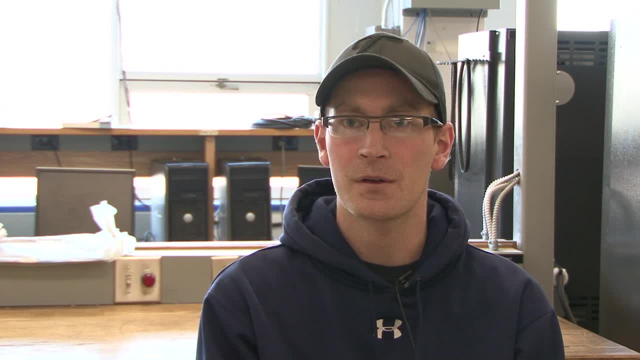 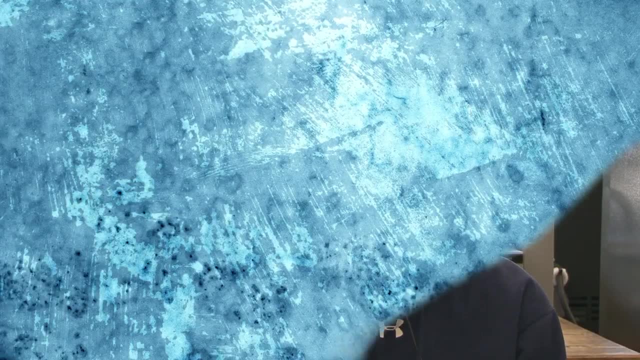